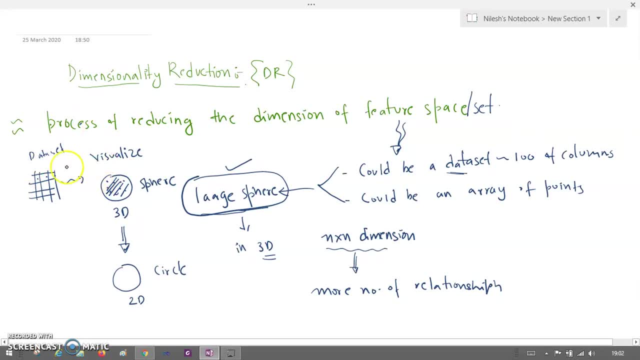 set. Then for visualization purpose, I need to visualize this complete data set which consists of n, cross, n. I want to visualize this. Then I can use something called a 3D structure. right, So for 3D I'm using sphere. So all these numeric values, the data points, I'm putting it. 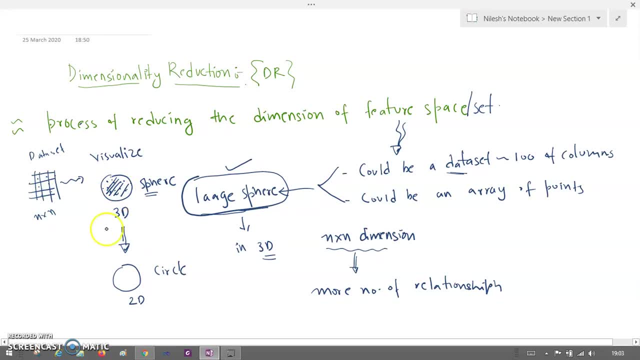 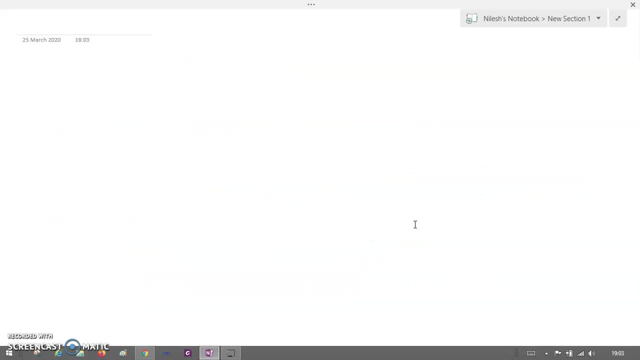 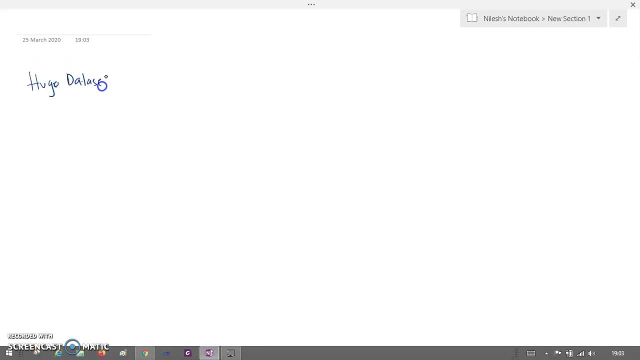 so if you are having a huge data set- let's say it consists of n cross n- then what will happen? Well, basically, if your n cross n data set is there, then definitely it is having more number of feature, more. 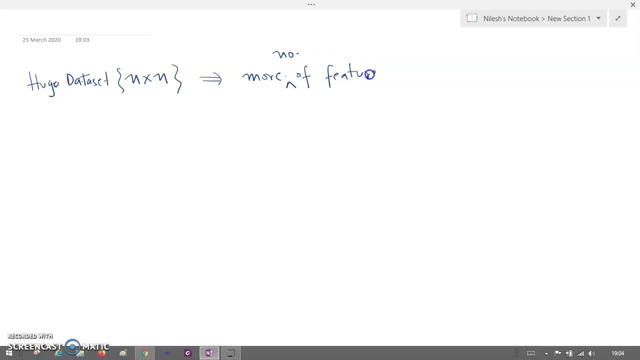 more number of feature. So if you're having more number of feature, then the model that you are creating is going to be very complex, is going to be more complex, Okay, And if you're- if there is, if there are more number of feature, then there is a slight problem to model it And 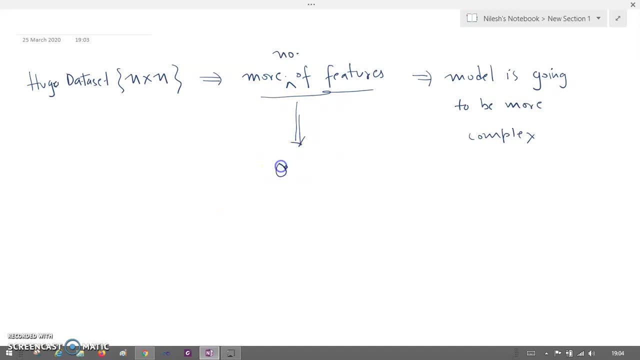 what is the problem Is? the problem is it will create an overfit model, And you precisely know why this happens. Well, this happens because you know that overfit model looks like this. If I have a data set like this you had seen in the linear regression, what will happen is I: 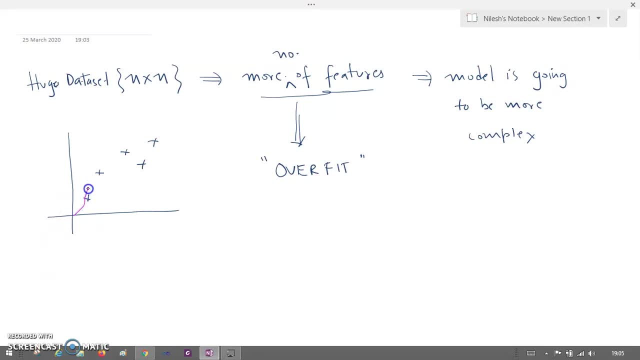 will draw a line which is going to be like: look like this It will. it will try to cover up all these data points and this, this is an overfit model. it is having the high variance and, because of this high variance, i have the overfit model. it will try to cover up all these data points. 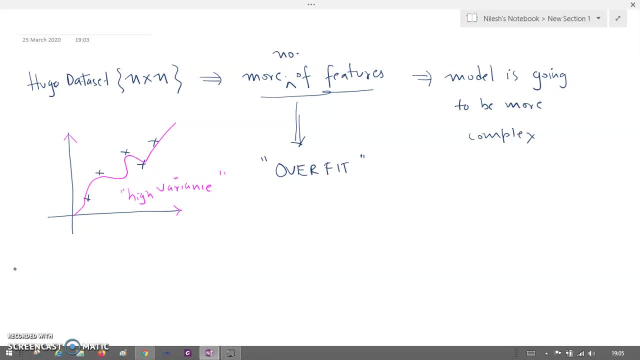 and it will generate an overfit model. okay, it learns from all the data set, from the, from all the data points, but the problem is it will create an overfit model and i don't need this overfit model right, because it is high, high variancy there. and what will happen inside the, inside the model? 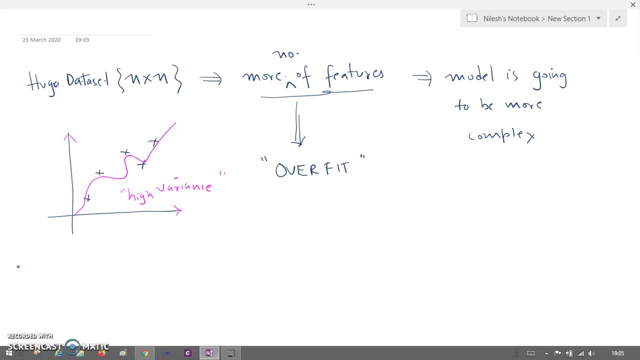 it will learn too much. that will not give you the. i mean it will always give you the good accuracy, always. there is no negative result in your data set. and i don't need that, because i need a result which consists of- i mean good result, i mean good accuracy, and also the bad accuracy, according to. 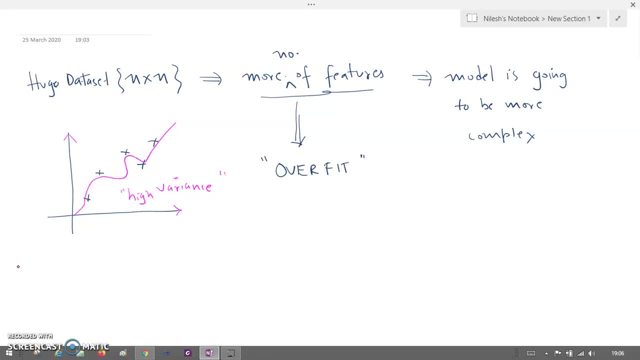 the data set. i need that kind of result, right. i don't need the best result. i need a very average result, that that consists of positive plus negative cases. however, this overfit model will give you only positive cases, always best result. i don't need it right. so that's why, if you are having huge data set and if there 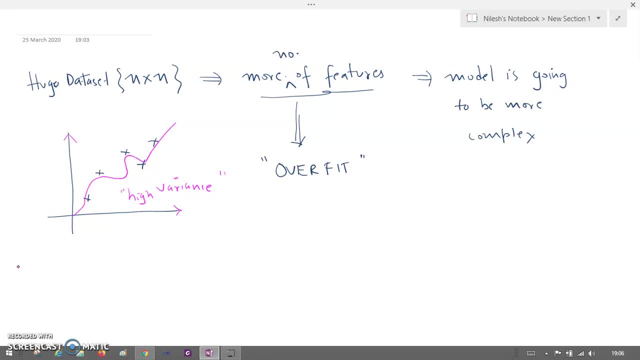 are more number of features then to to use that. uh, what will happen is the model is going to be very complex to understand. beside this, it will generate an overfit model, and i don't need it right, and that is the reason we are this: higher dimension to a lower dimension, with the help of dr. okay, so 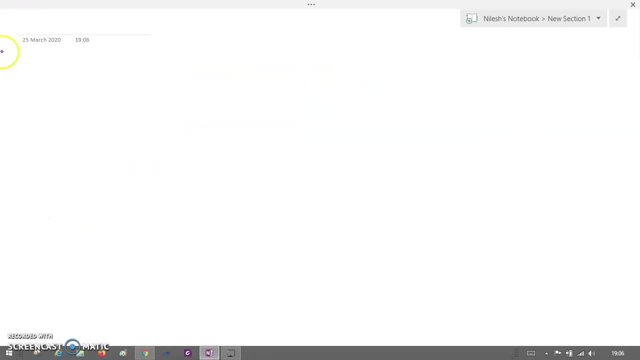 the first thing that we gonna do in dr is we will reduce and we will try to analyze and how to reduce a data from 2d to 1d and, by the way, this whole thing is from N to NG. so I'm thankful for the, for all these notes and the nice ended. 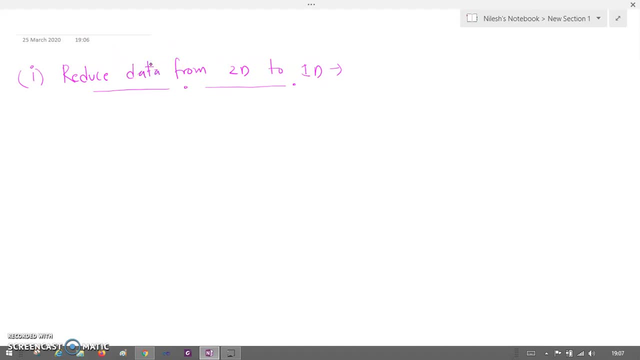 concepts. okay. so the first thing we can understand is how we can, you know, reduce this two dimension data to one dimension. so now, if you are having a graph looks like this- X 1 here and X 2 here- and my in my data looks like this: okay, so in linear regression, you know that I need a best. 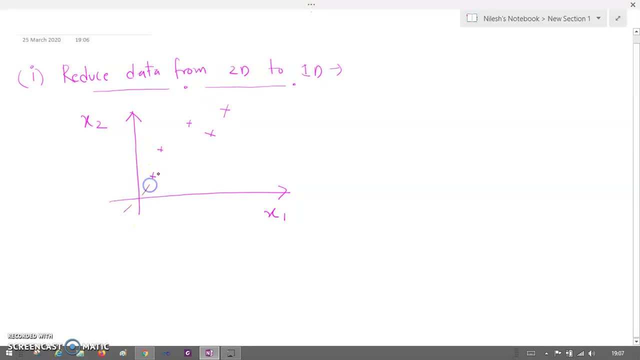 fit line and what I gonna do is I'll I'll create a feature space. this is the feature space. okay, so if I have this line, then what will happen is I need to project these. these data point to this line. I need to project it and how you. 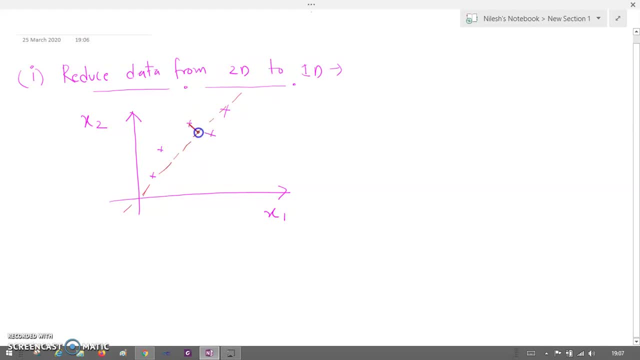 can project it. well, basically, you need a perpendicular line from the, from this line to this data point. you will project it. this is already there, will project here anyway. this is already there in the to the line. okay, so you are projecting your data point to this line and you try to minimize this, minimize this distance. so 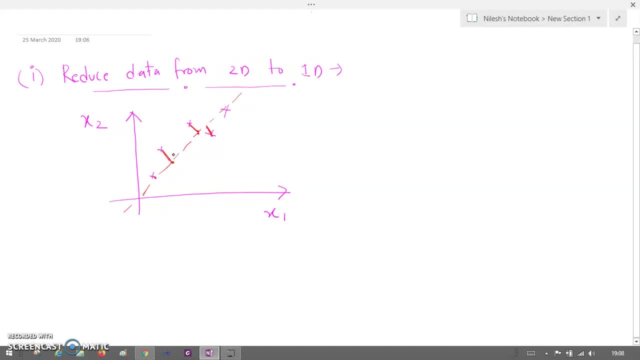 that you get you know, so that you got some reduction in your dimension and by means of projection you understand it. projection is nothing but in the data set. if X 1 is 0.5 and let's say X 2 is like 0.9, and if X 3, 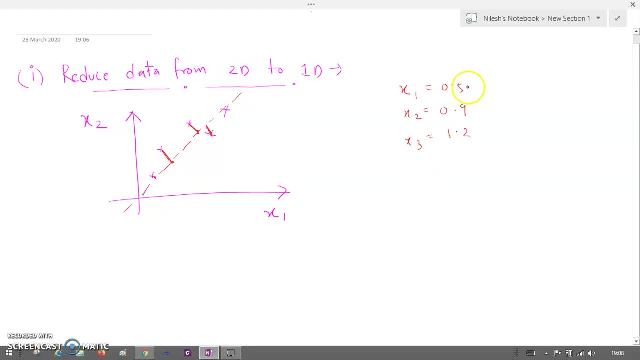 is going to be like 1.2, then what will happen is this X 2 is basically very near to 1, okay, and this X 3 is also very near to 1. so what will happen is this: if this is, if this cross is, let's say this cross is, let's say, X 2, okay, and the point. 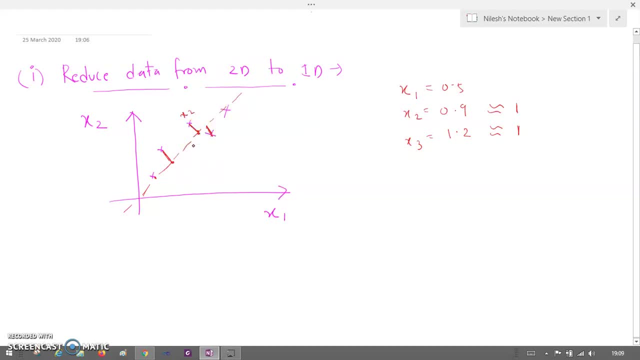 that is there very near to this line is, let's say, X 3, and you can see X 2 is 0.9 and X 3 is 1.2. then what? what I want, what I want to say for project projection is basically is that I can take this X 3 here instead of X 2. I'm I'm just 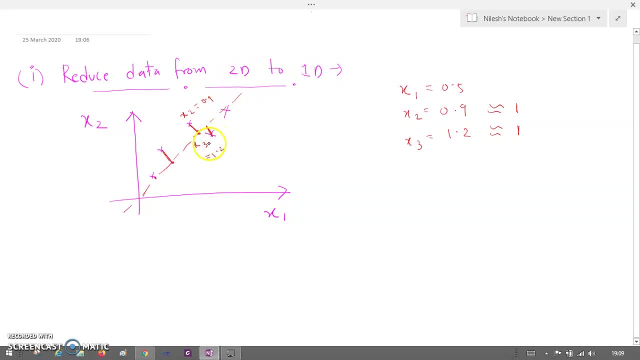 projecting it. okay, so I'm converting this 0.9 to 1 and I'm seeing this 1.2 as equal to- I'm sorry, approximately equals to 1, so what I'm doing is, instead of using X 2, I'm using X 3. now, okay so? so what is happening over here is from the. 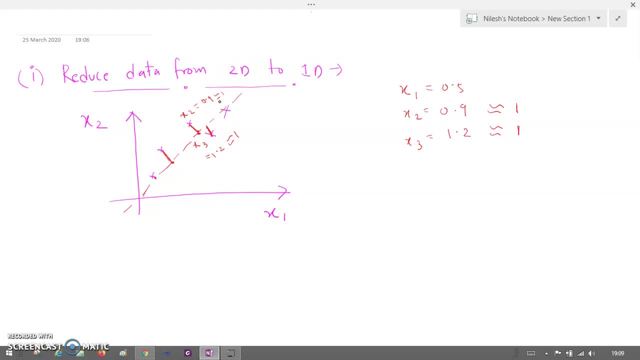 from the independent variable. I mean these X 1, X 2, X 3 are. I mean they are independent variable. so I'm creating new independent variable here. so this X 2 is my old independent variable here. this is my old independent variable and this X 3. 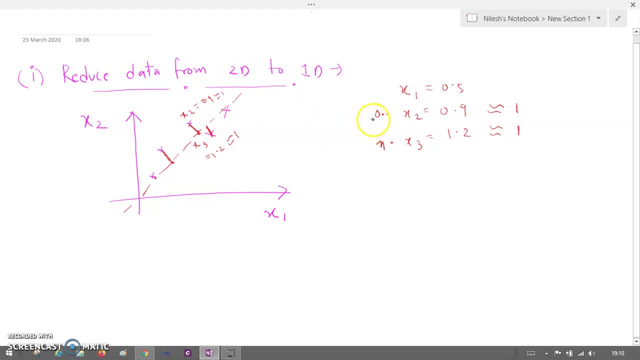 is going to be my new independent variable. I am projecting this X 2 to X 3 because their values are same, so I can use that right, and their values are very nearby. so that's why I'm using X 3 here. okay, just for you know, just for to get. 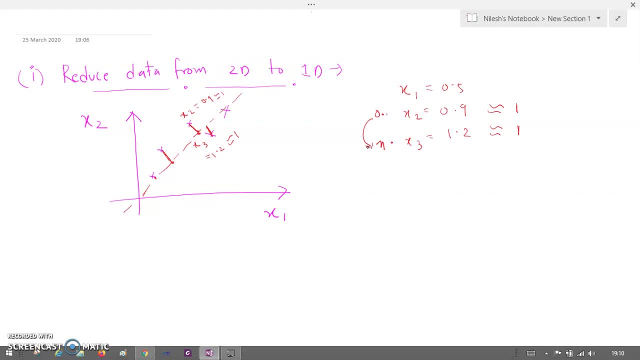 an idea on projection. I'm just explaining in this way. it is not happening in real. in real scenarios, however, just to understand projection, it is nothing, but you are taking the nearby data point, which is very near to the older independent variable. so if X 2 is 0.9 and is equal to 1 and X 3 is 1.2, then it is also equals to 1, so so I'm. 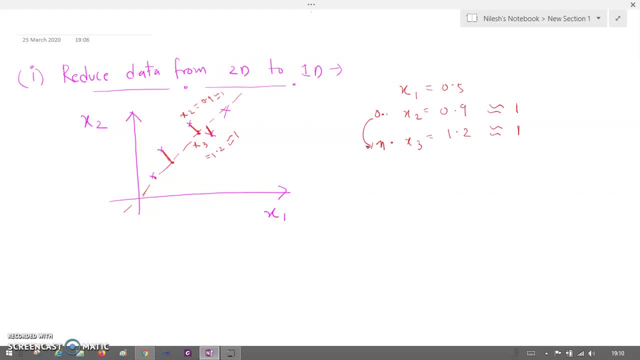 projecting my X 2 to X 3. so now X 3 is going to be, you know, represent X 2. okay, so the projection meaning is like that and the intention is now the. this is in 2d. I want to convert this in 1d. so what I'm going to do is I'm going to do is I'm. 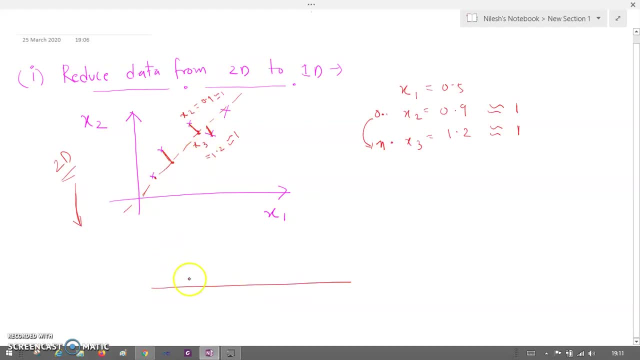 going to take this line. I'm going to take this line and I will say these, these points. I will take these points and drawn it over here. so this is so. let's say: if this is, let's say this: this is X 1, this is X 2. let's say: this is let. 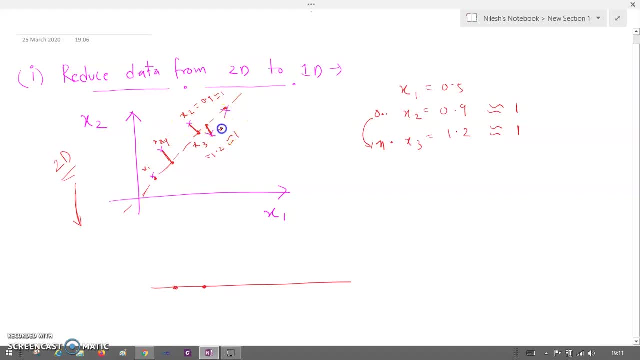 me take it as: this is X 4, this is X 2 and this is X 3 already and this is X 4. okay, So what will happen is: this is my x1 here, x2 here, x3 here and x4 here. 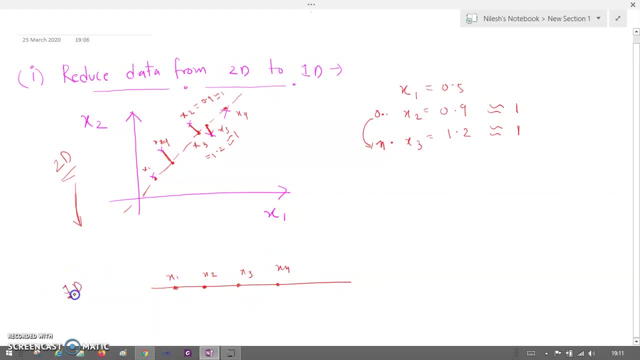 And you can see this line is in 1D, So initially it is there in the 2D dimensions. However, now it is converted into one dimension And I will not use this x1,, x2, and x3, and x4.. 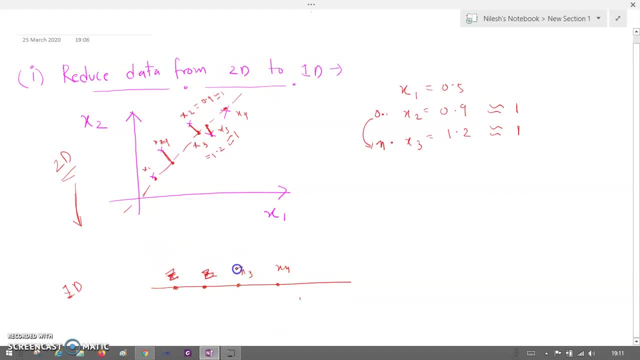 I will use instead z1, z2, z3, and z4, instead of using x1, x2.. So what will happen is if my x1 belongs to 2D now because of this projection, because of this projection, it is now in the 1D. 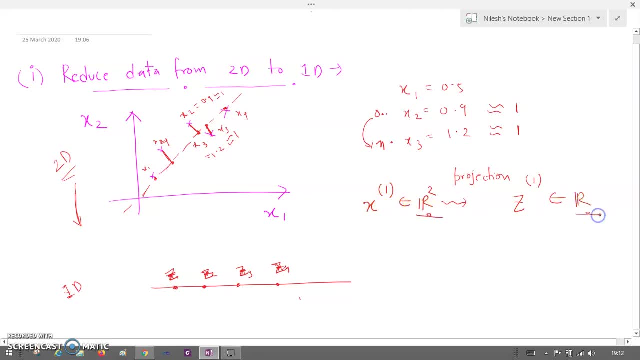 So initially it is in the 2D, Now it is reduced to 1D. In the same way I can write it for x2.. It belongs to 2D Now because of the projection it is converted into, or you can say it is reduced to 1D. 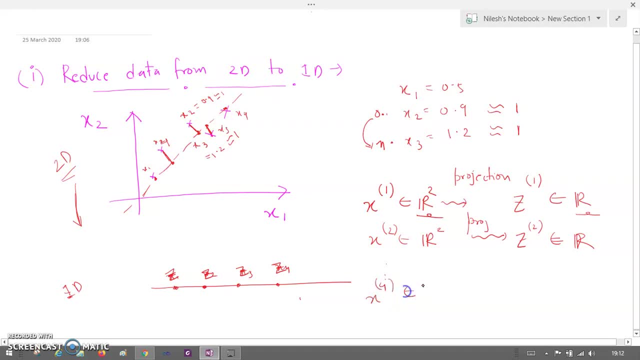 In the same way you can write for x4.. For the projection: for the projection, this is 1D. Okay, Are you getting it So? initially it is there in the 2D, Now it has been converted into a 1D. 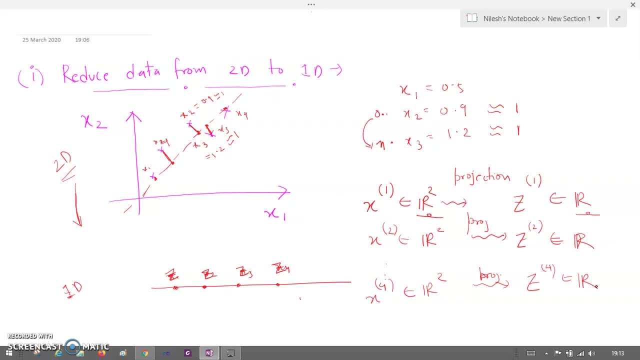 And what will happen if I do that? Well, you can have an idea over here, So I'm going to scroll it a little. So what will happen is because of this reduction, what will happen is: you will, you will. it reduces, it reduces the memory space. 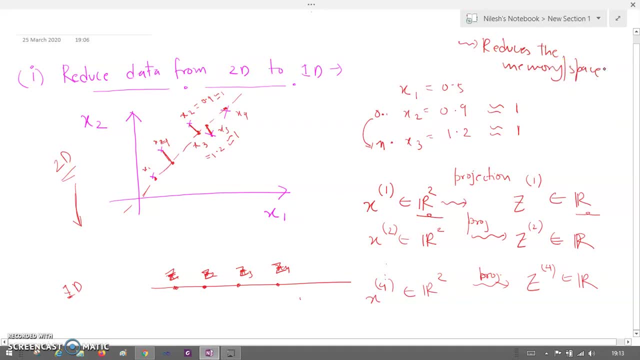 And you can easily understand it right. You can see earlier, it is using two dimensions. that and because of that reason it uses more number of features. Now I am, you know, reducing it to one dimension, for 1D only. 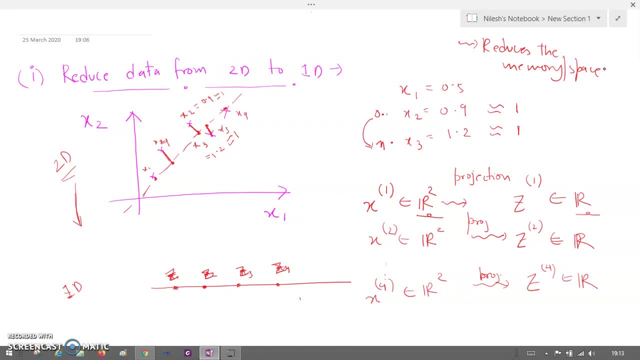 So I'm, I'm, I'm using, I'm using a very little memory from the, from the computer. Okay, And based on. if you are using less memory, then definitely the second advantage is it runs quickly. Okay. These are the two things that happen if you reduce the dimension of the data set. 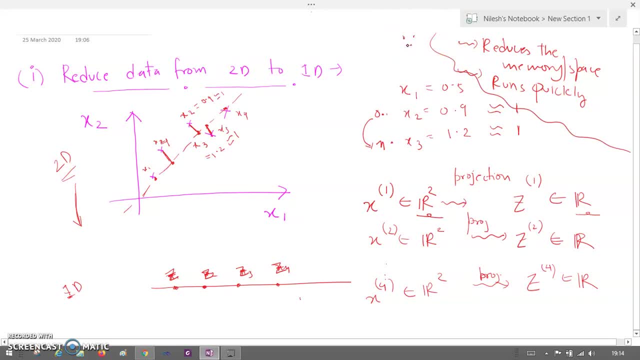 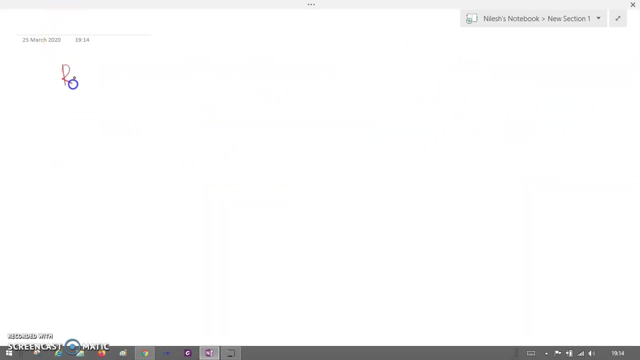 One is it reduces the memory space. as you're dealing from a higher dimension to lower dimension, you're reducing it. And the second advantage is it runs quickly. Okay. Now, the second scenario is you are converting or you are reducing. you're reducing 3D, reducing your data. 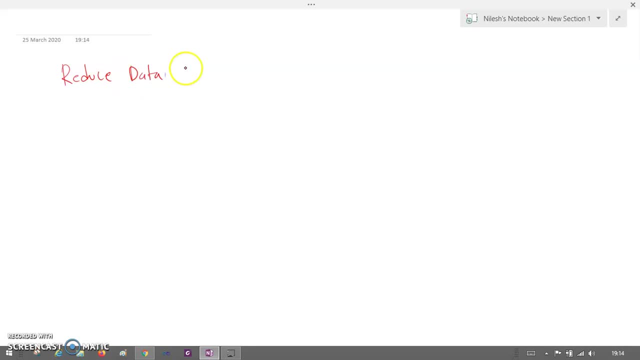 Let me just reduce data. Okay, Reduce data from 3D to 2D. How we can do that? Well, basically, if you're having, I'll try to draw it. So, if you are having like this, so this is 3D, this is going to be my x1, x2,. 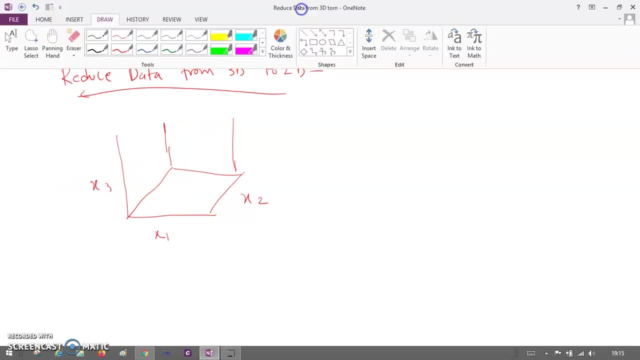 and this is x3.. And for data point, I'm going to take another color. So so these are the, these are the my, these are my data points. I hope you can see this. So all these are data points in three dimension. 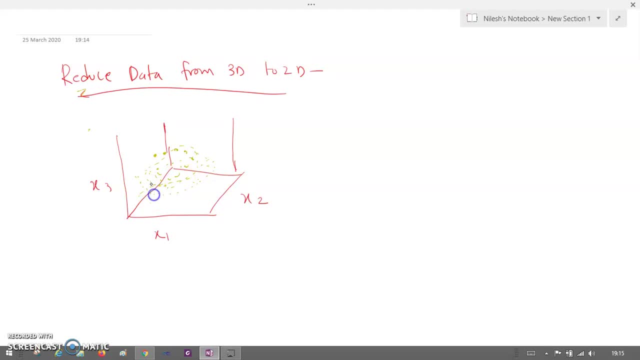 They are not counter lines, They are just randomly scattered, Scattered here and there in three dimension. Okay, I want to convert this whole thing into the three dimensions. Sorry, in two dimension. So how can you do that? Well, I'll write it over here that my xi. initially it belongs to three dimension. 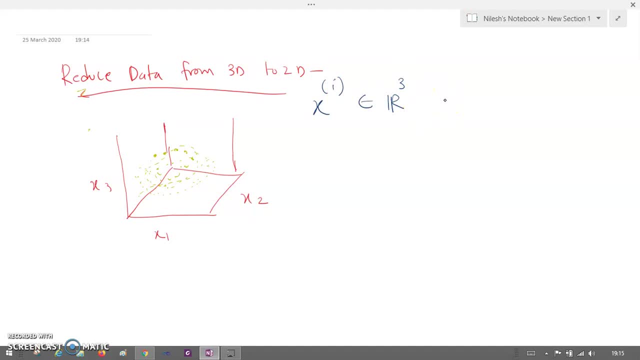 And I want it to convert into the two dimension. So what you can do is you can take one. you can take one plane over here. It's like a. it's a 2D plan, So it's it's actually a plane, just a plane. 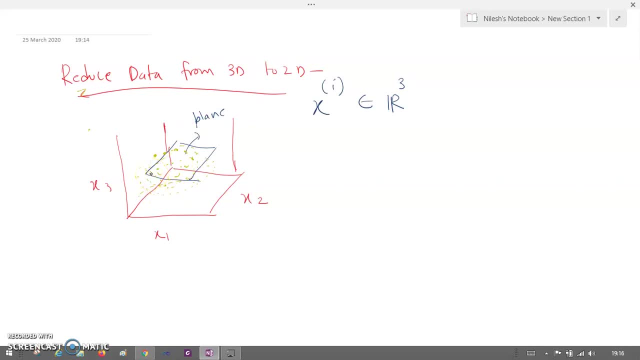 This is the plane And you are just, you know, slightly, you are just moving it Slightly, you are moving it for the 2D. So now I'm, I'm, I'm just changing this graph to, so I'm projecting it. 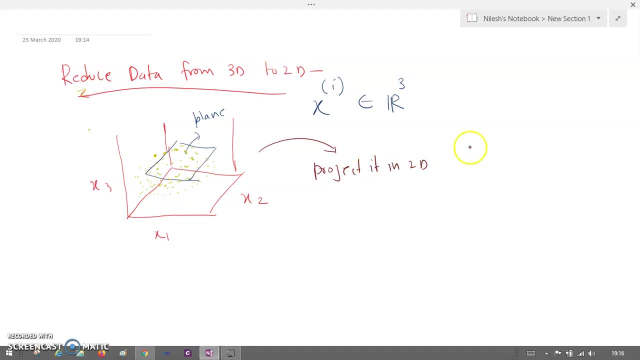 Project it in 2D. So what will happen is I'm going to draw it again. So now what will happen is these: so I'm going to, I'm going to tilt this plane a little. So now, this is the. 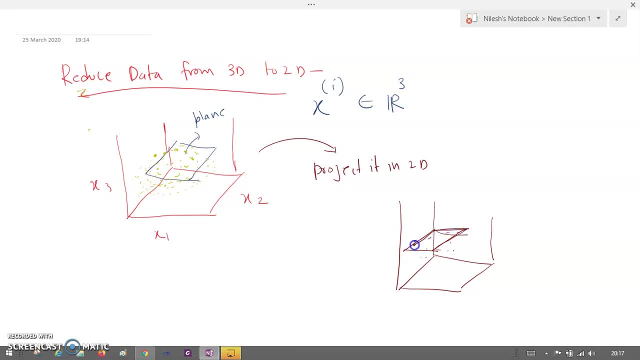 I cannot draw it, But this is the tilted version of this 2D plane. Okay, And initially here there are three, three dimension. to to show this three dimension, We're having X1, X2 and X3.. And I plotted two dimension. 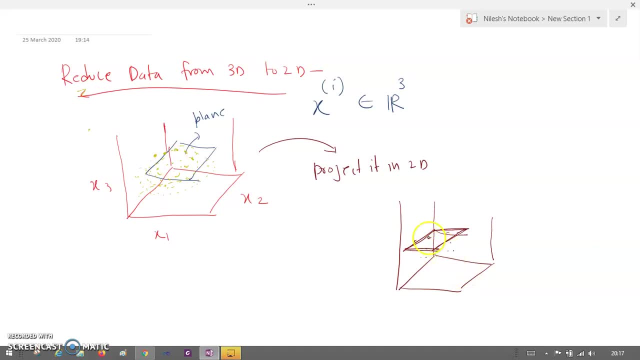 sorry, 2D plan. I tilt it a little And this is original X3, X1 and X2.. But now the the data point which is there inside this 2D plane, happen is. I need here two dimensions. 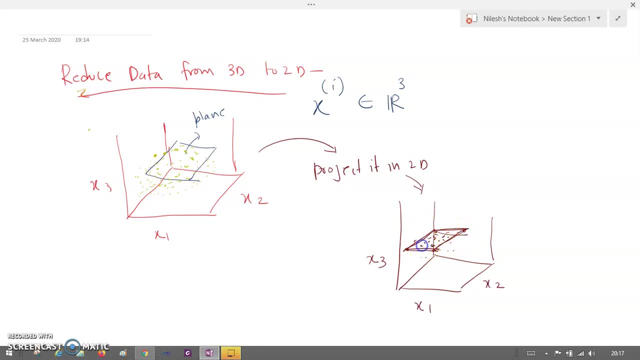 Okay, Basically I need two dimension to to see these data points, So I need another two dimensions. So these are my two dimension. I can represent this dimension as Z1 and Z2.. Okay, These are my extra two dimension, not extra. but 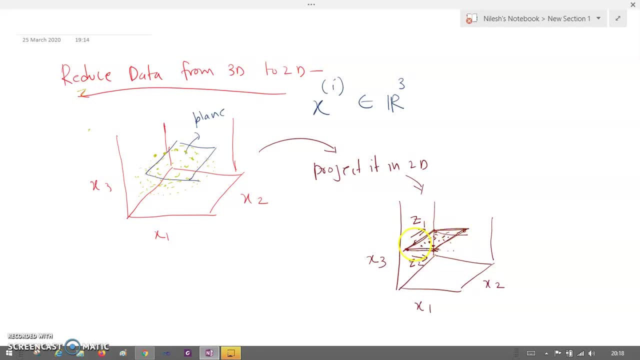 these are the two dimension by by which I can see this 2D plane And when I take this out, when I take this out 2D plane, I can show it in in this way And I can have these. 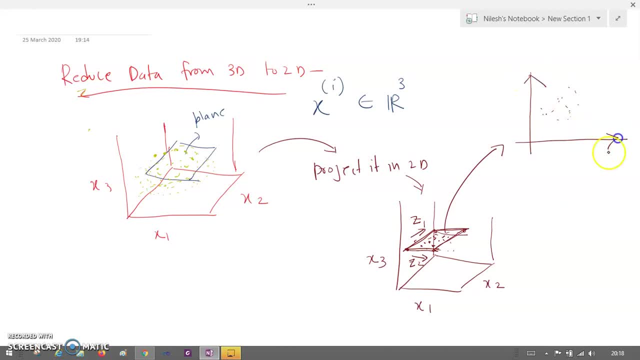 these all data point besides over here. And so this is the graph for Z2 and Z1.. Okay, So, initially your here, initially your XI belongs to three dimension, But with the help of projection, you know. now you are representing this. 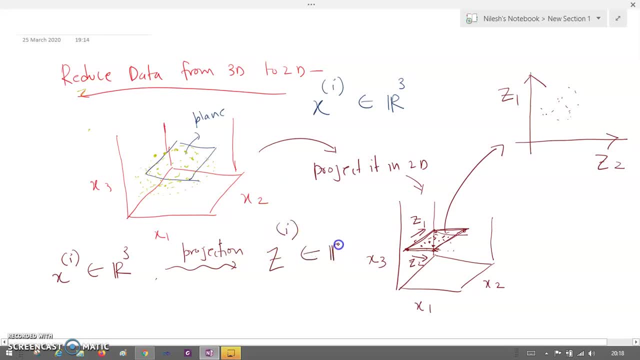 the form of Z, Z of I, And it belongs to two dimension. This is what we are seeing inside this topic. So this is your dimension reaction and we precisely had seen how to convert this 3D to 2D. 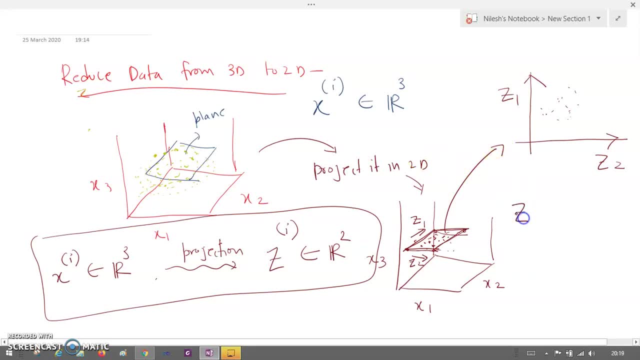 And you can see this whole Z it is consist of here. we have two Z because we are dealing with two dimension. that's why the Z is the vector space. Z is a 2D vector space. Okay, I hope you are getting it. 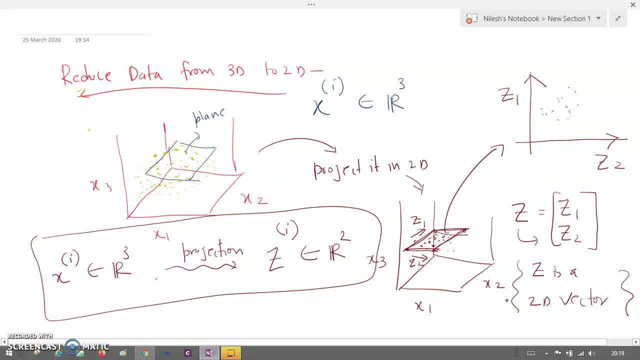 So this is your dimensionality reaction and we precisely use to reduce the dimension from data cells so that we get fewer relationship and the model becomes simpler and easy to understand, And we we ignore the fact that we have over fit model. 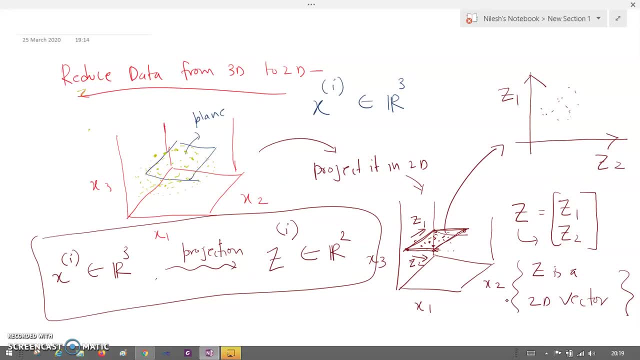 Okay, We convert the over fit model to a good model with the help of reducing our dimensions. So this is the the complete set, or the complete idea on dimensionality reaction, And you have varieties of application to do that We have. 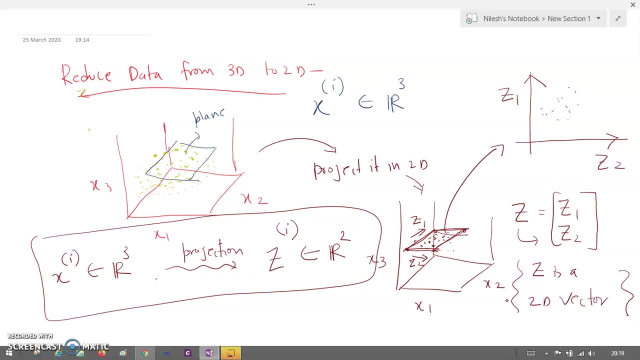 we have principle component analysis, PCA, that is the. that is our next topic that you can see where we can apply the the same thing, this feature extraction, And we will see how to reduce the dimension from higher dimension to lower dimension with the help of. 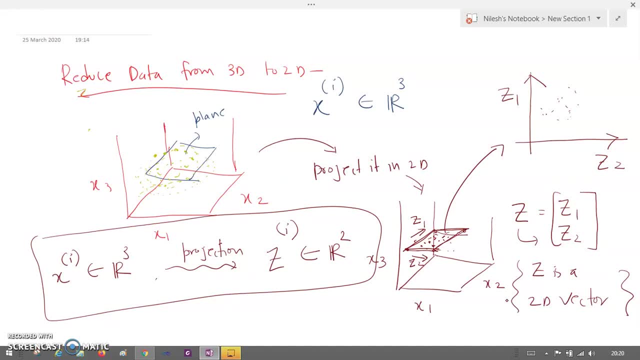 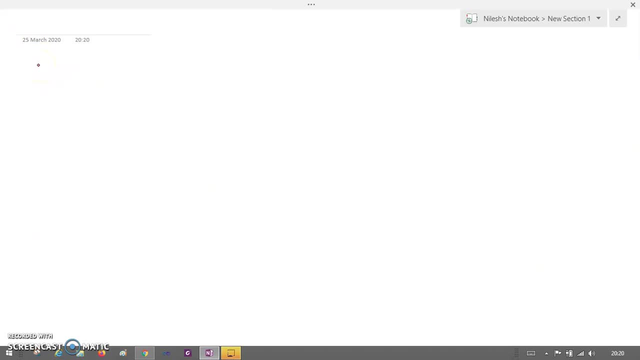 PCA, Now TR can be. you know it is. it can be. as I told you that, how can I, how can I use this TR? How, what are the various methodologies by which I can apply it? So there are. 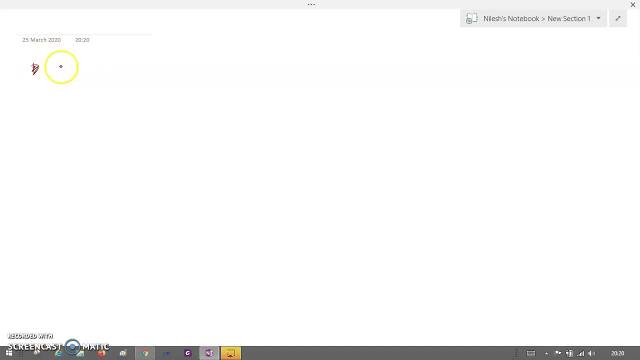 three method. actually, there are two methodologies: One is linear method and the another one is non-linear method. We are dealing with linear methods over here, So this is your linear method. Okay, So this linear method consists of: 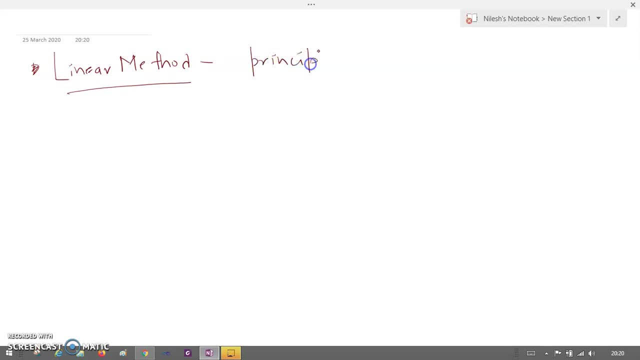 first one is principle component analysis. This is principle component analysis. This is PCA. Okay, As I, as I told you and you can take this, you can have a look on this, on this topic, in my next. 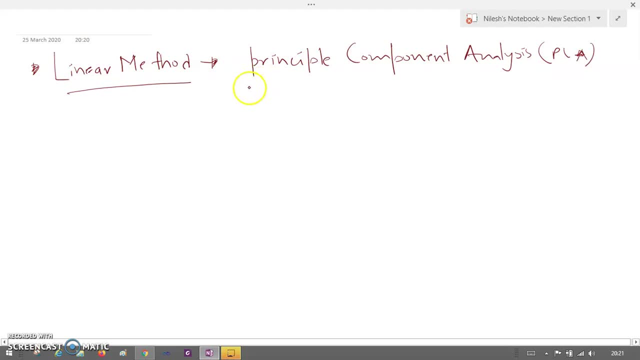 you know video So I will not elaborate this PCA all over here. in this video You can check it out, that video where I explain you what is principle component analysis. So please go through that. refer the next. 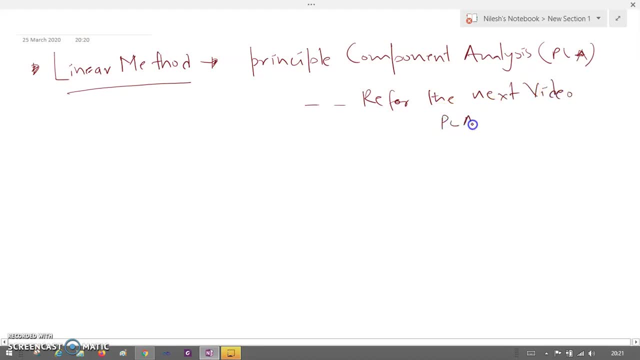 video. Okay, Refer the next video on PCA. So this is done. The next thing is we can use something called as factor analysis. Okay, We have this topic- factor analysis- by which we can use, by which we can reduce the. 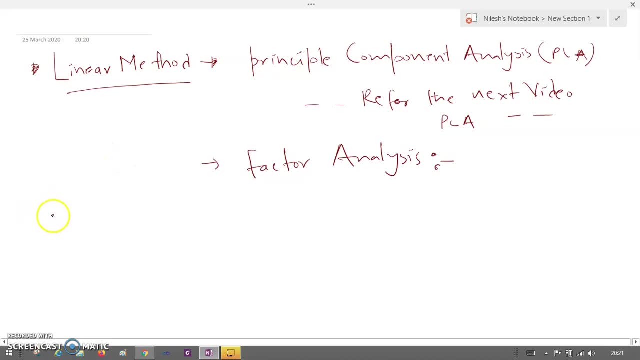 dimension D And how it can be used. So it's factor analysis says that you know we are having something called as observed variable. I will say they are. they are some set of variable which are 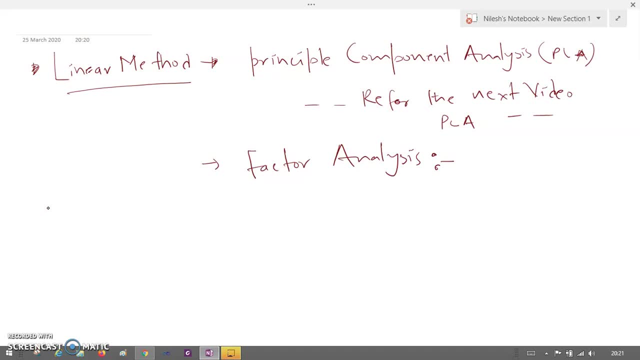 which look similar. They have the same similar characteristic. So instead of using five different name for the similar characteristic, I am using one, one specific name for that. Okay, That your factor analysis will give you. So. 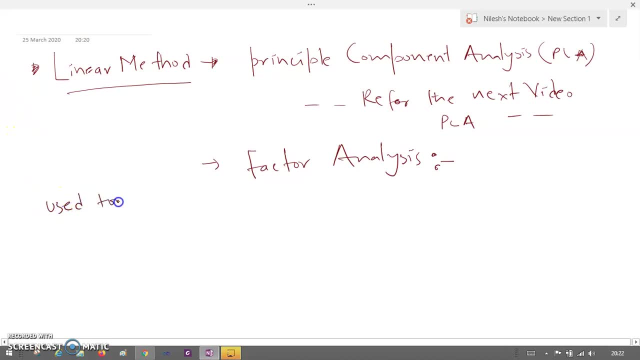 what it says? it says that it used, it used, it used to reduce a large number of. it used to reduce a large number of variable into fewer number, As I told you, fewer number of factors. 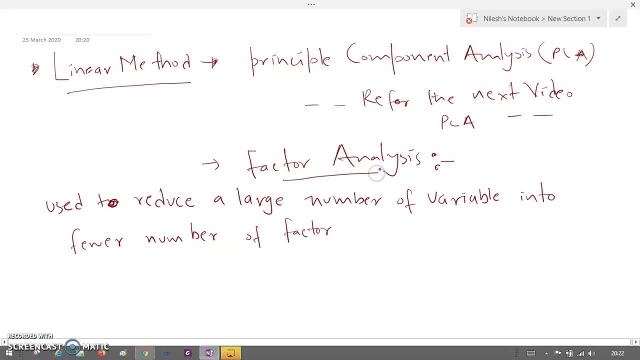 So what it means? it means that five variables are having the same characteristic. If five variables are having the same characteristic, then I will not use five different name. I will not use five features, Okay, Instead of that. 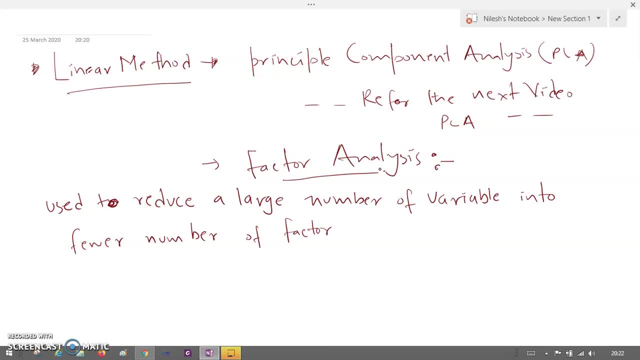 I will use one feature to represent that five feature. So if let's say, if let's say, I have length Okay And I have width Okay In the data set, Let's say: 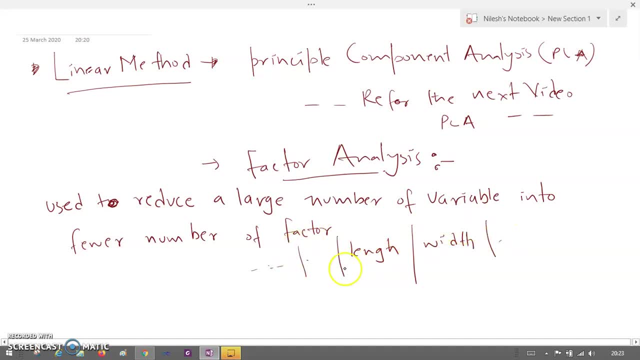 all other columns are like this: Okay, So if I have length and width in the data set. So instead of using two different feature, what I gonna do? I will simply say: area equals to length. 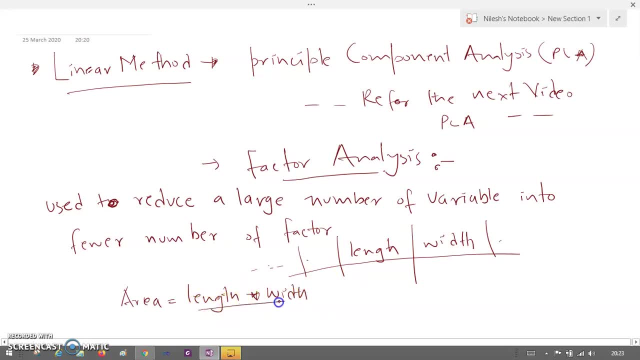 cross width. So now, instead of using two different features, what I gonna do I will simply use one feature only. So, instead of that, what I gonna do I will use simply area. Can you understand? 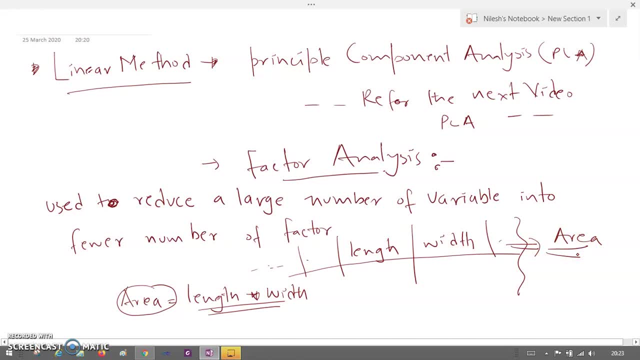 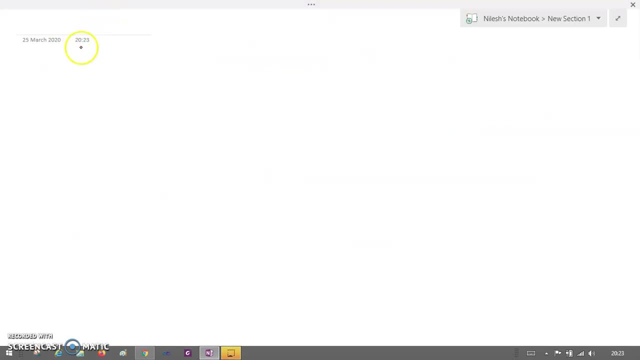 So the exact thing factor analysis will give you. Okay, So I'll write it here. So the example is from one website, So I'm just putting those example here. So if I have observed variables, 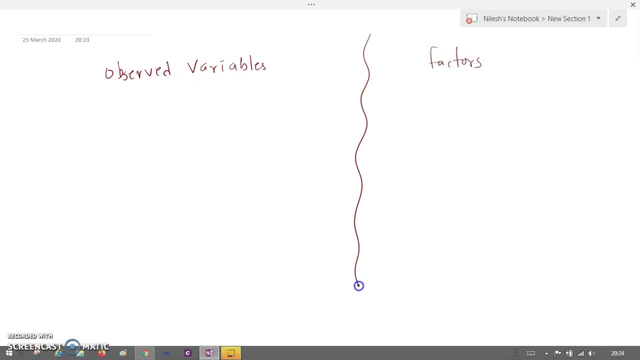 and the factors I'll represent over here And let's say, observe, observe, variables looks like this: If I have, let's say, let me just change this. Let's say, I have taste of food. 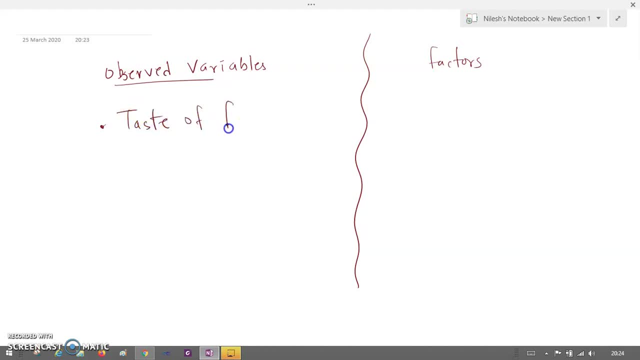 This is one feature. Another thing is, let's say, I have food temperature, Food temperature. I'll also say freshness of food. Okay, And you can precisely see that these, I have this, this. 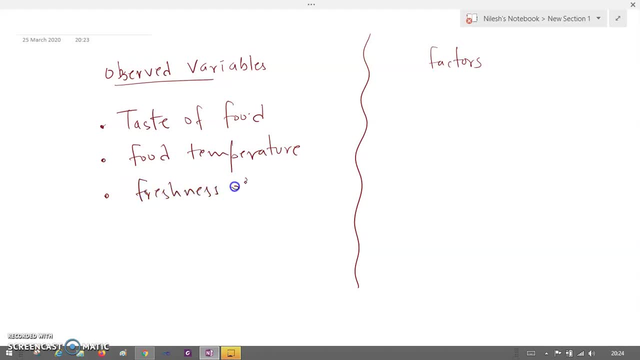 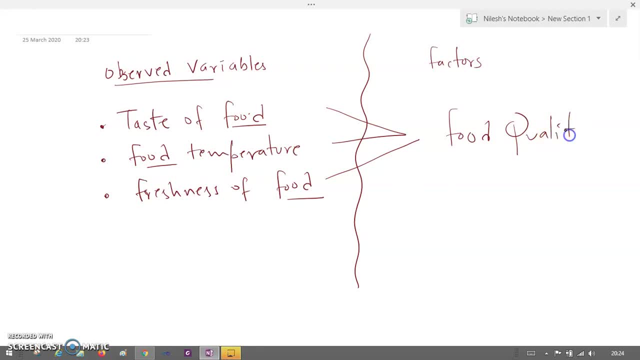 And that feature name is food quality. So you you have to take one equation or you can say one expression by which you can, you know, represent these three observed variable into one. So 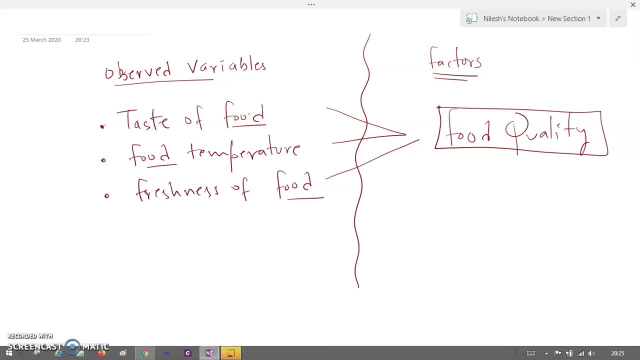 I'm using that one variable, using here only one feature. okay, this is this exact thing will give you. it can be done with the help of factor analysis. okay, and the third and the last most thing: in the linear method for dimensionality reduction, it is the LDA. 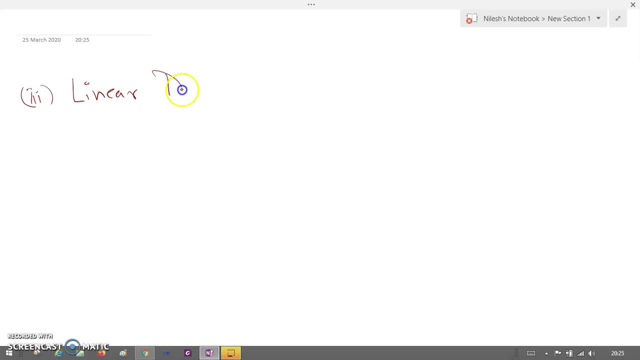 and I'll say linear discriminant analysis, shortly abbreviated as LDA. so what it says, it it is. it looks like this: so you can put the- you know, same data points having a similar characteristic into one- I shouldn't say cluster, but you can put all those data points who are possessing? 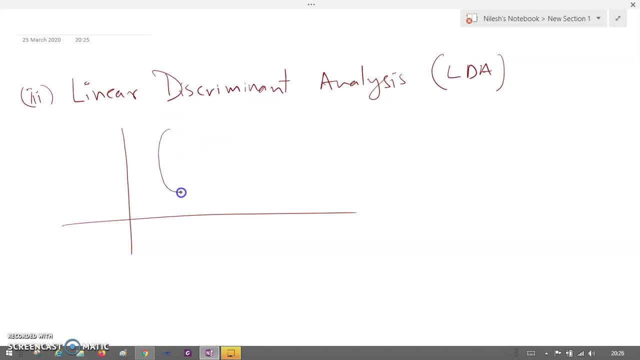 a similar characteristic into one bunch. so if this is one dense, then I am putting those crosses over here, because these crosses represent the similar characteristic. another bunch is for these round shaped, you know, points who are having the similar characteristic. so this is it. look, it's something like this in the in general, this is my ld1 and this, this set here. this is the complete. 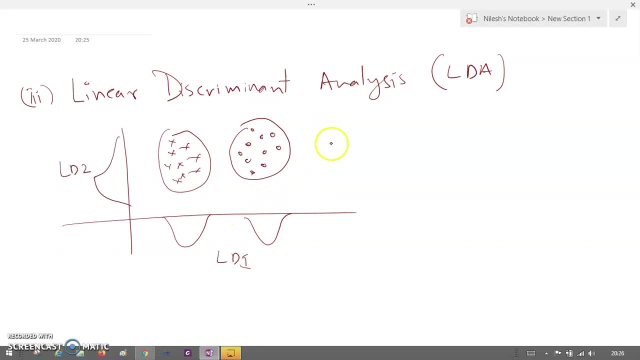 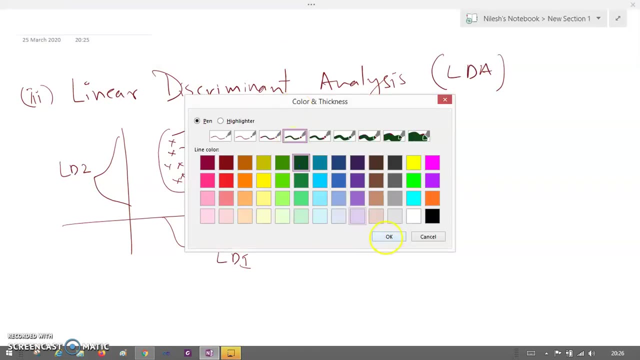 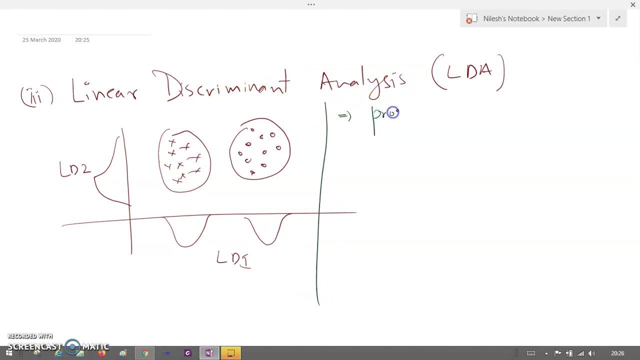 thing. this is my ld2, okay, so what is it? i'll? what is the definition? i'm going to change the color again. so what lda says? it projects the data, it predicts the data in a way that class predicts the data. that is, class separability is maximized. okay, so your class separate separability gets maximized. so we are we. 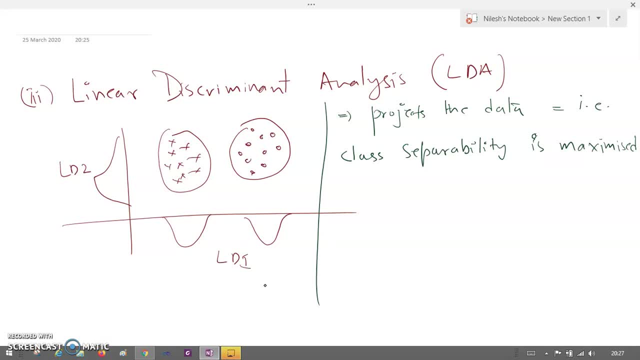 are projecting the data in a way that the similar characteristic data get into the one bunch, the, and there must be a proper separate separability between two bunches. okay, that is, we can see over here: this is ld1 and ld2 and you can see there are two different classes. okay, and having the 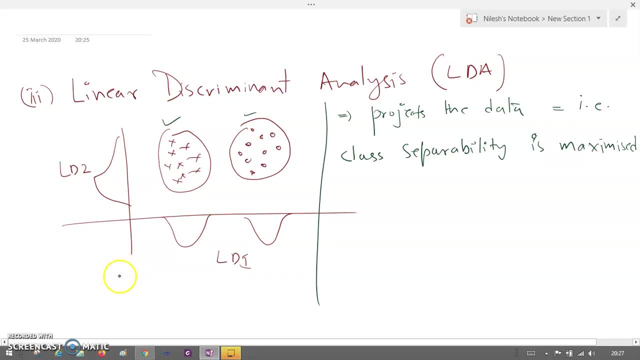 different, different characteristics, but inside one bunch. they're having the similar characteristic examples from same class put close together. so i'll write it. i'll write it down here: examples of same class. so these cross are the examples of same class and examples of same class put together. 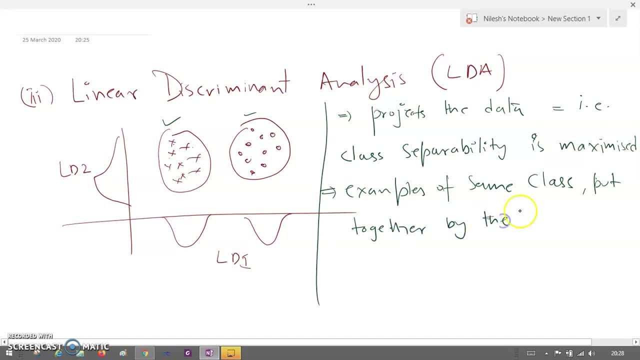 put together by the projection and, as i told you, the projection means uh, as i told you, x1 is having 0.9 and x2 is, let's say, 1.1. then both are very near to one. so i'm putting these x1 and x2 into. 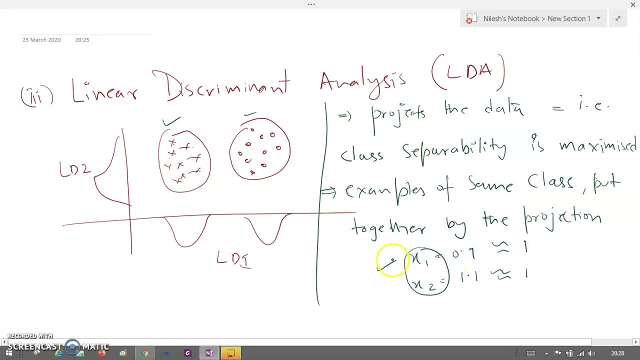 one bunch. okay, this is the. this is the thing that lda do, and the other thing is the opposite. the different classes are. so if i have a space here, so i'll write it down here. so i'll write it down here. different classes are, so examples of different classes are placed far apart. 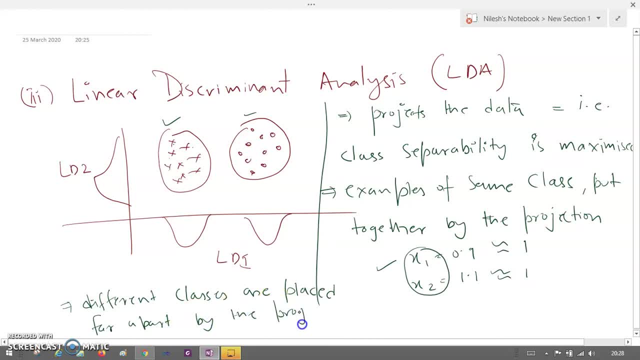 by the projection. okay, so this is the thing that we had, uh, that we had seen in the dimensionally. these are the. these are the three methods. these are the three linear method by which you can use the r. okay, so, principal component analysis, vector analysis and we have linear discriminant analysis. 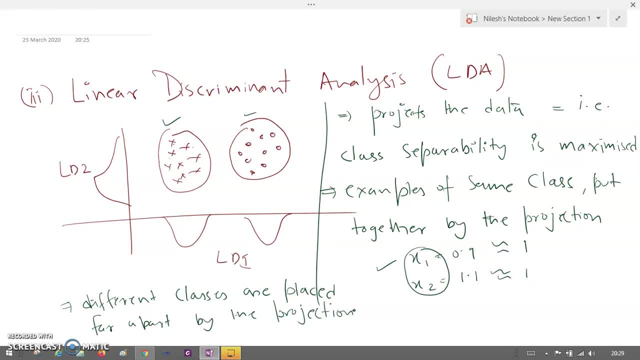 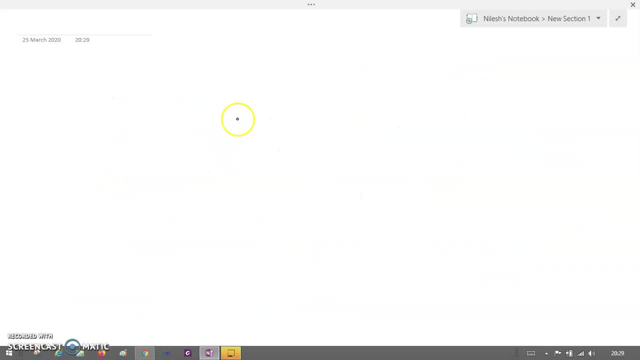 okay, these are the three methods by which we can uh use a dr. we can reduce the dimension from higher dimension to uh lower dimension. apart from that, also, as i told you, for the, for the projection. so, again, i'm just want to conclude something. so, if these are the data points and and if this is the 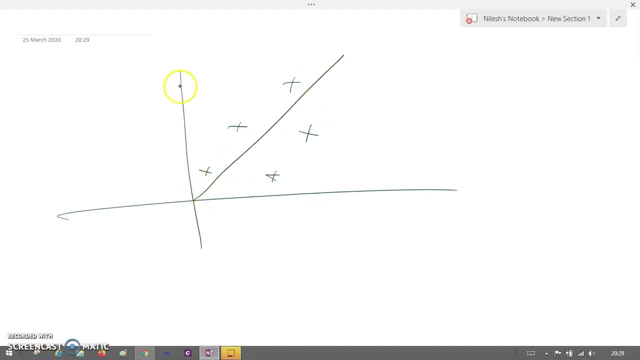 line, then what is the thing that you need and what you need in order to be able to, to generate the value of the Texas do in the dr? well, basically, if this is the graph, so if this is the graph, then you draw a line like this to have your projections. okay, so if this is the projection, then, uh, what will happen is: 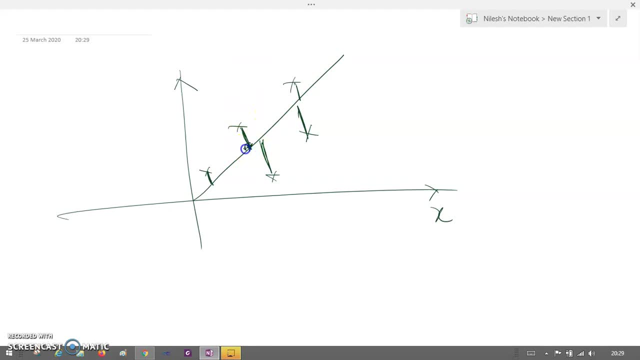 so you are taking this point. so these round shaped are going to be the projected data. okay, cross and round shaped, cross and round. so here cross x or you can say the cross represents actual data. however, the cross with circle is going to be projection of actual data. 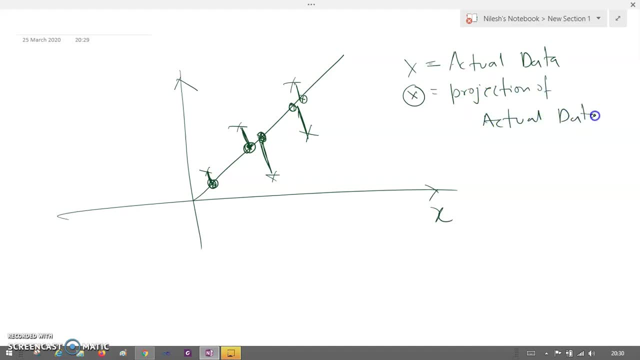 okay, so this is what we are seeing here and this is the best projection why this is the projection of the actual data. okay, so this is the best projection. why this is the best projection? because the error is a minimum. this is the minimum distance. this is also- uh, you have to take care that.